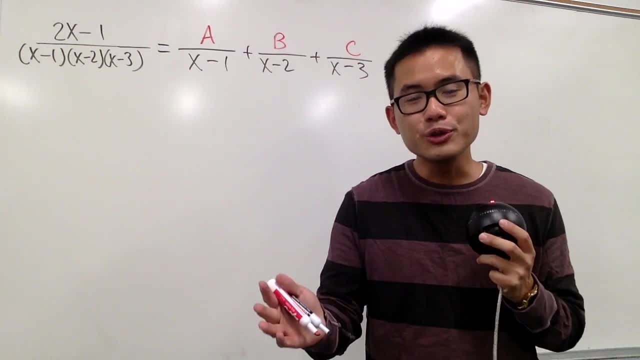 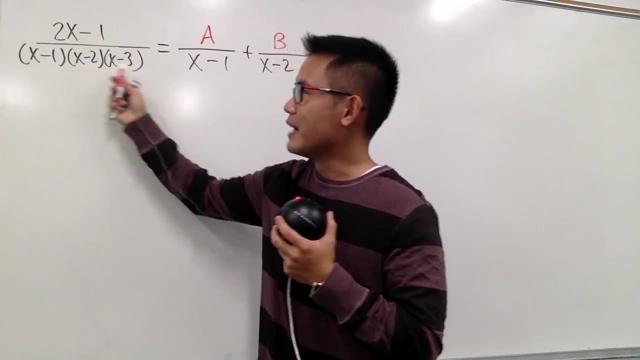 I'll show you guys how to do the partial fraction with the Kavra method and I'll also show you guys why it works. Here is the rational function that we want to break it apart. As we can see, we have the denominator to be factored in already, right, So that's great. 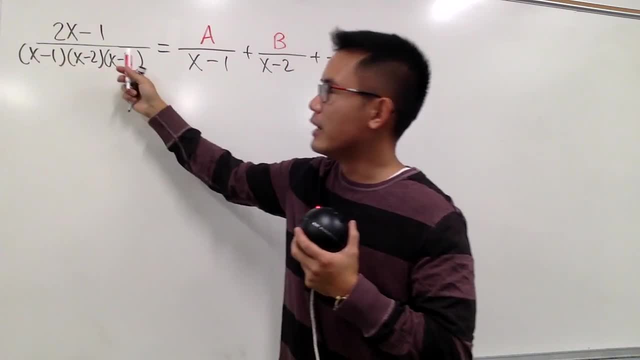 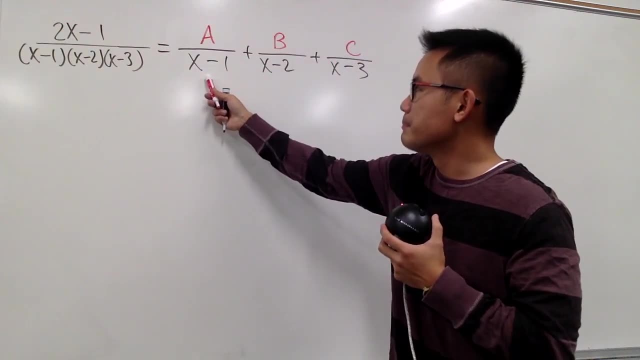 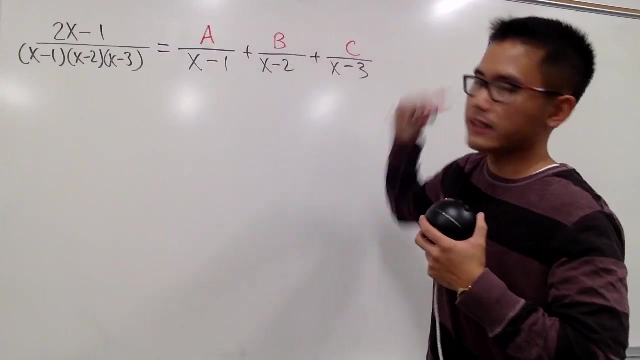 2x-1 on top over x-1, x-2, x-3.. So the setup is because they are all linear and they are all different. you just break it apart. It's x-1 here plus x-2 right here and then plus x-3, with a constant a, b, c on top, like that. 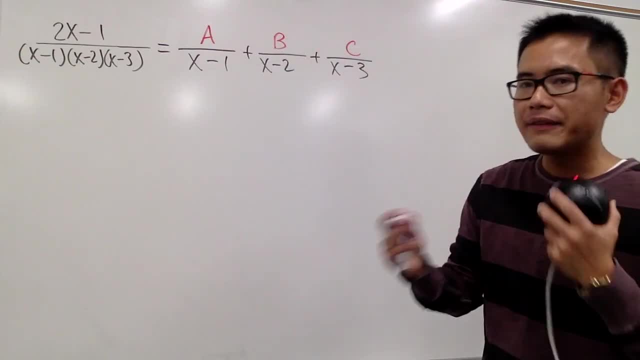 Our goal is to figure out what are the values for a, b, c. After that, we'll be done right. Okay, so maybe you're watching this for pre-calculus class or maybe you're watching this for your Calc 2 class. 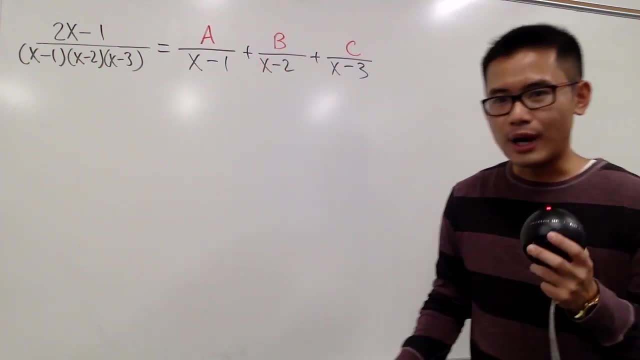 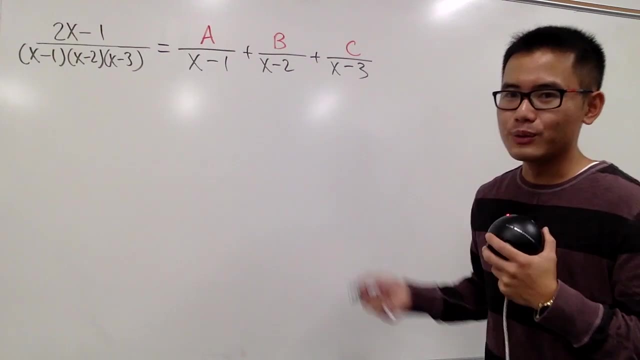 For pre-calc, you can just figure out the a, b, c and you're done For Calc 2, after this you start to do the integration. okay, But anyway, our goal is to figure out the a, b, c values. 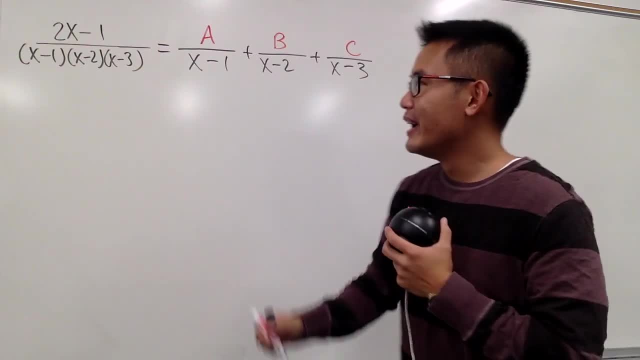 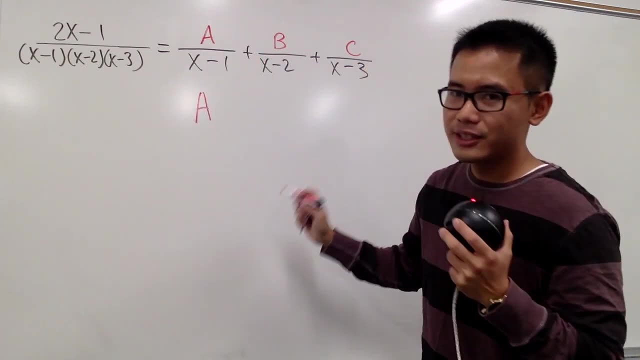 And this is how. First of all, let me just show you the magic Right here. if you want to figure out a, this is how you can do it. Let me just write it down for you guys already: a. it's going to be the following: alright, 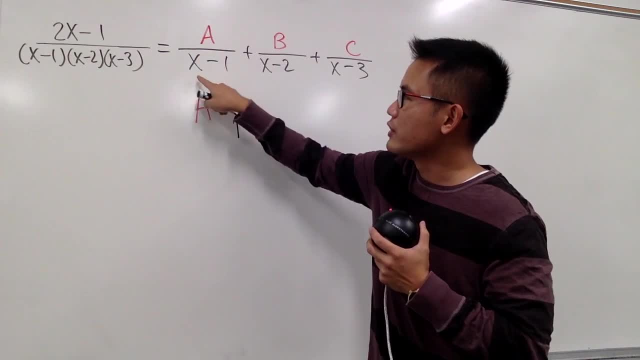 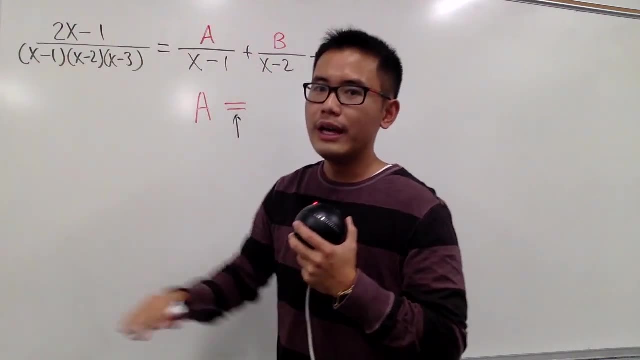 So, as you can see, a this fraction here we have the denominator is x-1.. So what you do is you go back to the original and use your other hand, right, So just use your fingers. maybe I'm going to cover up the. 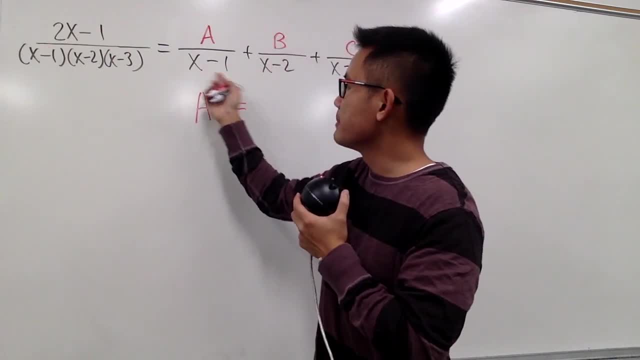 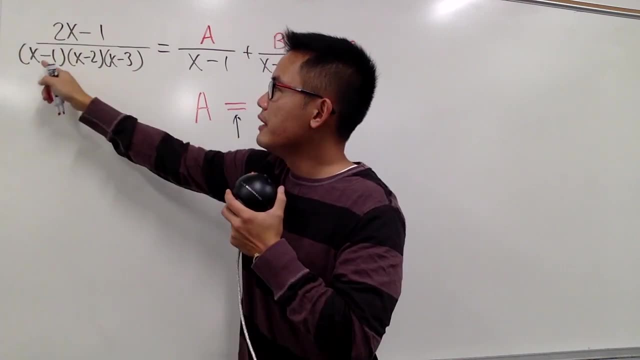 The same denominator, namely x-1,. right, This has x-1, we cover this up as well. And now you're going to ask yourself: how can you make this factor equal to 0? This is x-1,. x has to be what. 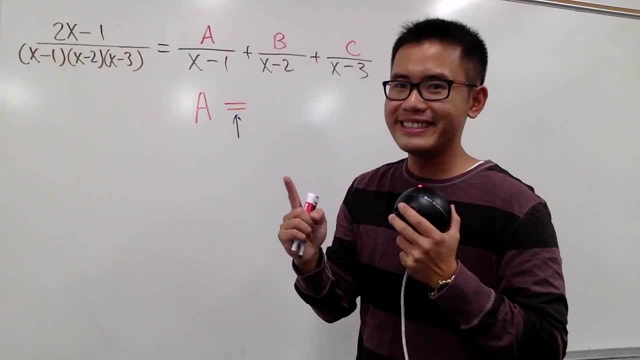 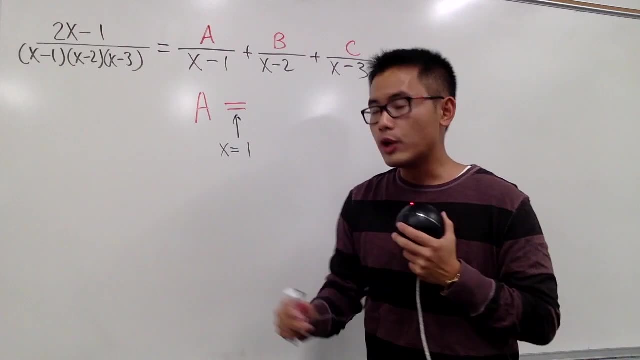 So that this will be 0.. x has to be 1, isn't it So? with that being said, a is going to be x is equal to 1.. What we'll do is we'll plug in 1 into the remaining x, right here, alright. 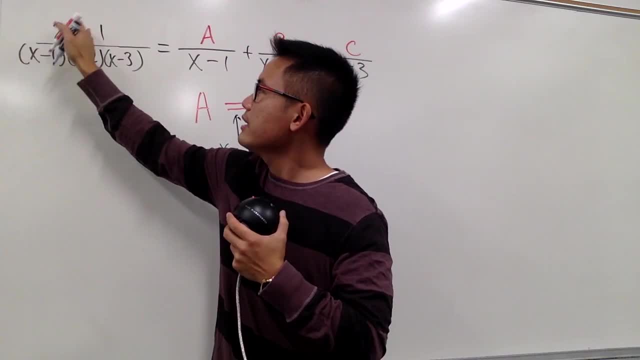 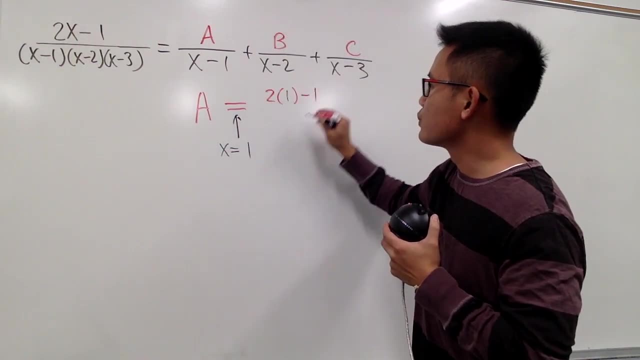 Because we covered this up And now on the top we will have 2 times 1, minus 1.. And let's write it down: 2 times 1, and then minus 1, over. Since we covered this up already, we don't bother with it, alright. 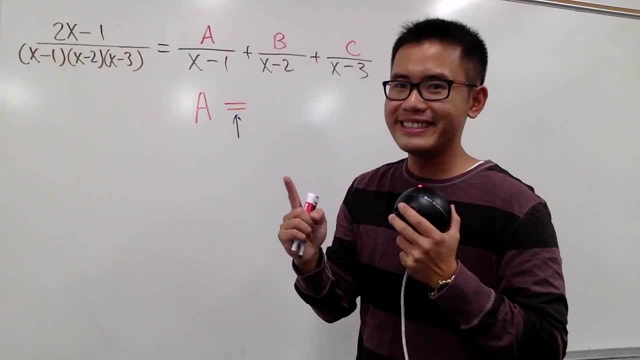 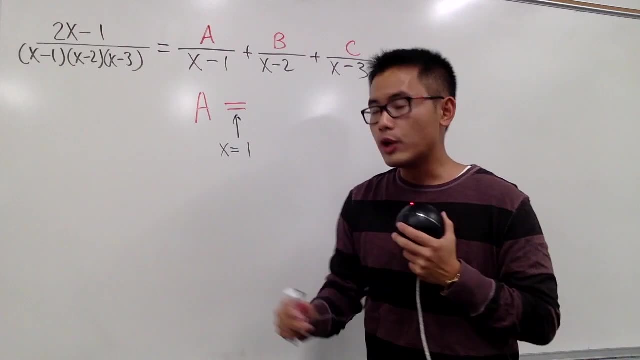 So that this will be 0.. x has to be 1, isn't it So? with that being said, a is going to be x is equal to 1.. What we'll do is we'll plug in 1 into the remaining x, right here, alright. 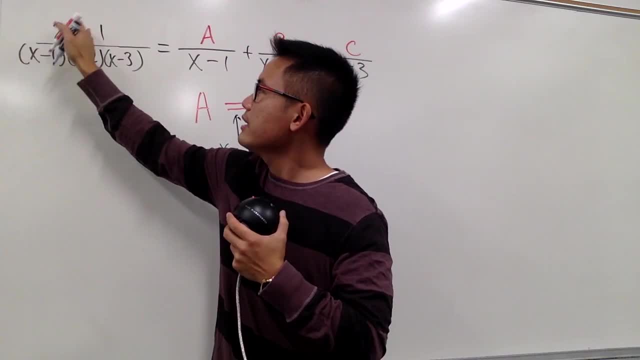 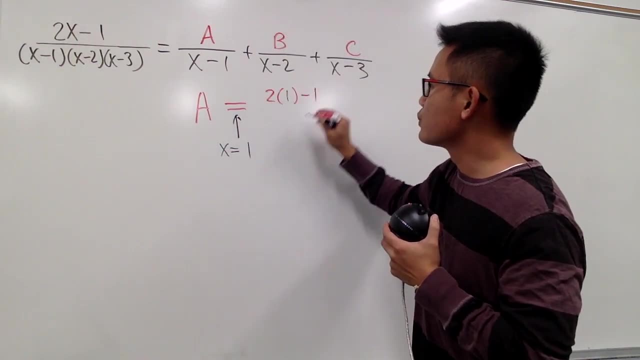 Because we covered this up And now on the top we will have 2 times 1, minus 1.. And let's write it down: 2 times 1, and then minus 1, over. Since we covered this up already, we don't bother with it, alright. 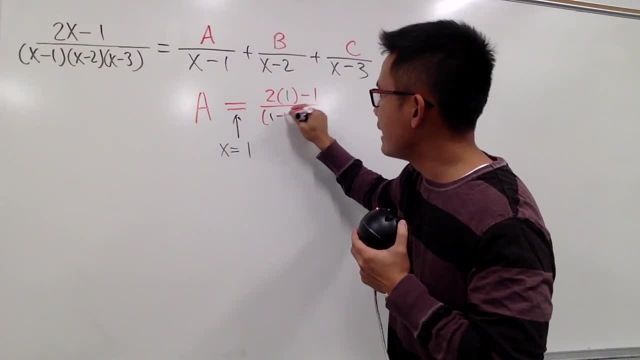 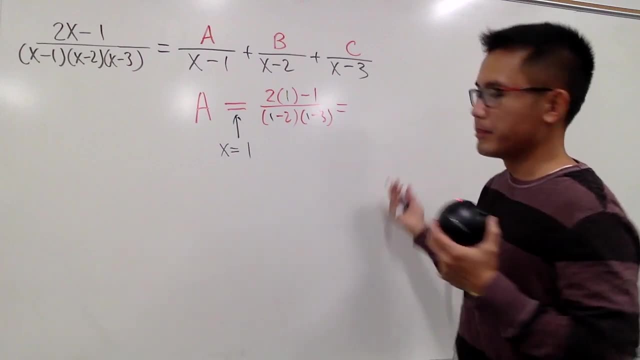 We're plugging 1 into here, so we will have 1 minus 2.. And then we're also plugging 1 into here, so we have 1 minus 3, like this, And then just do the computation. 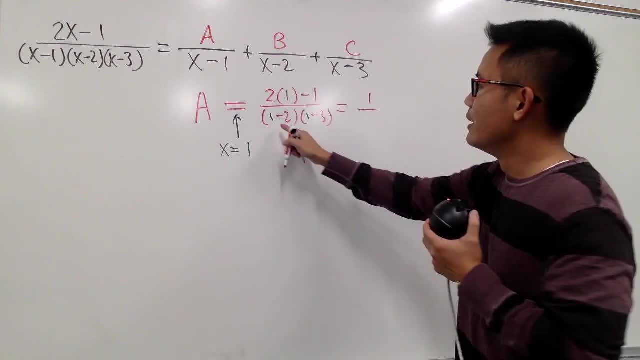 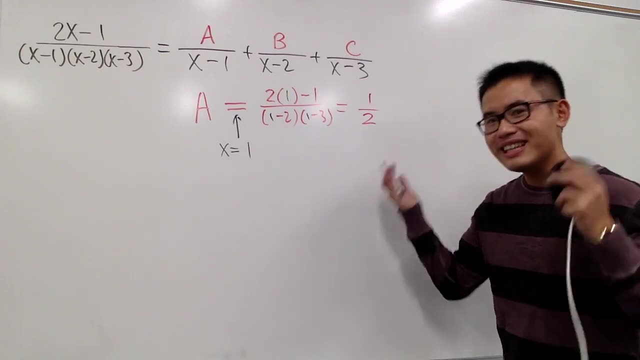 2 times 1 is 2, minus 1 is 1.. Over this is what? Negative 1 times negative, 2.. So all together, it's going to be positive 2. And that's it. That's the magic right. 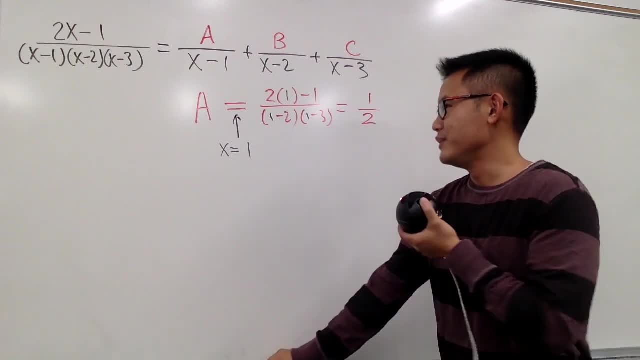 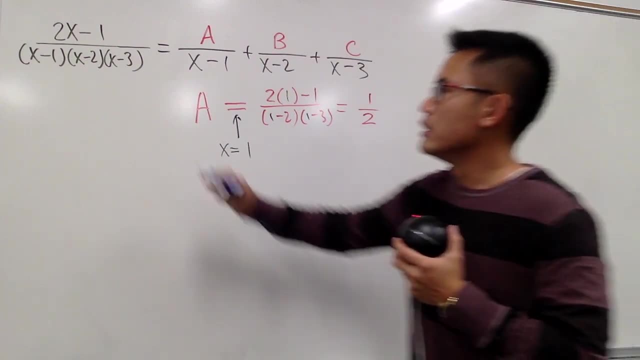 And now let me show you guys why it works. Of course, if you see this, you can also do the same for B and C, But let's just use A as an example. What we'll do is: this is a rational equation. 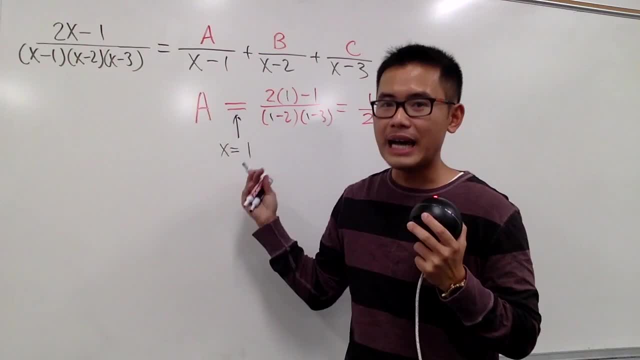 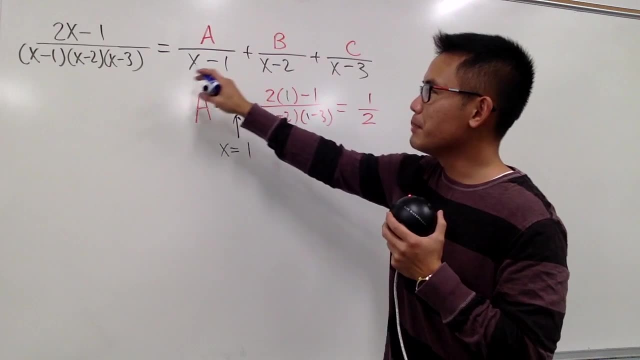 Usually we have to multiply everything by the lowest common denominator, namely all these three factors. But Let's be smart. We are just going to multiply everything by this denominator, namely x minus 1 only. So let me do that right here for you guys, alright. 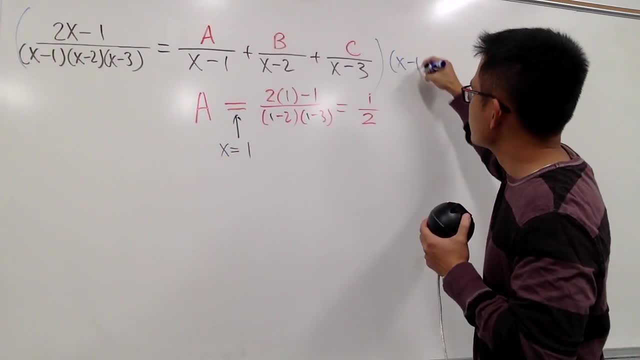 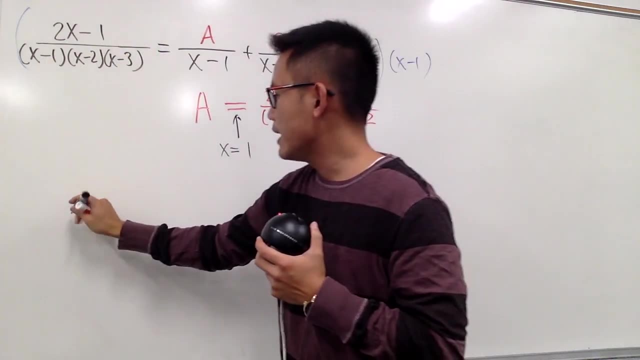 So multiply everything by x minus 1.. Just this. And now let's see what do we have This times? that We will just have 2x minus 1, over this and that cancel. That's why, as I told you, it didn't matter. 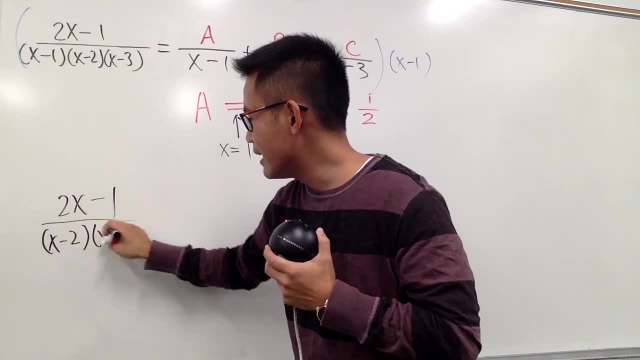 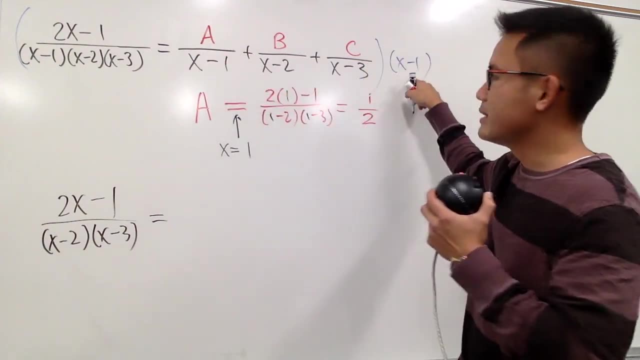 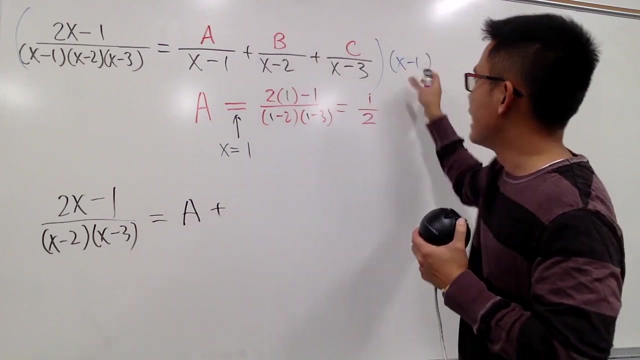 We will just have x minus 2 times x minus 3 now, isn't it- And this is equal to well, this fraction x minus 1 times this they cancel out. so we have just A and plus. well, this times that. 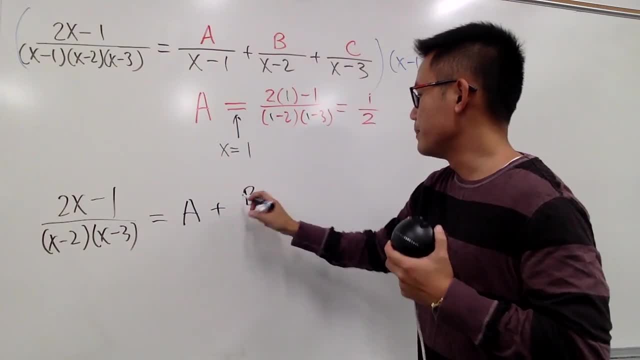 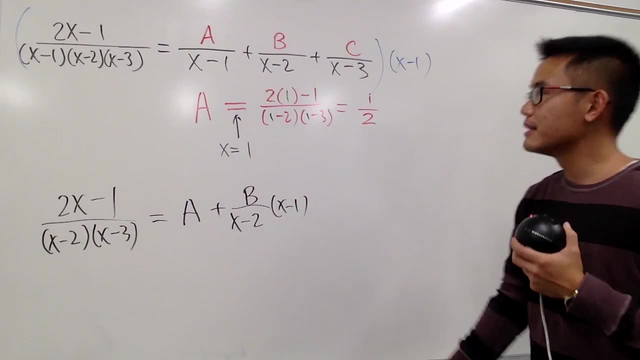 I will just put this on the top right, So we will have. well, just let me write it down: It's B over x minus 2 times x minus 1.. I don't want to multiply anything. alright, Once again for this right here, same thing. 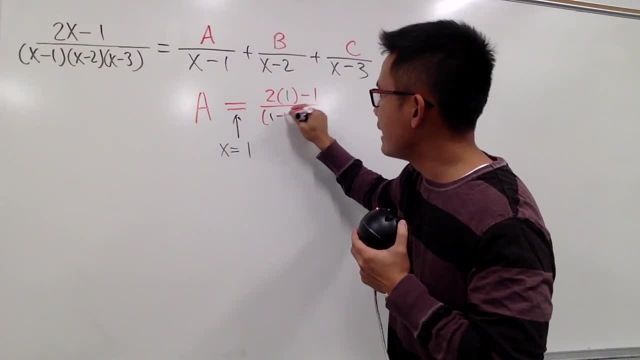 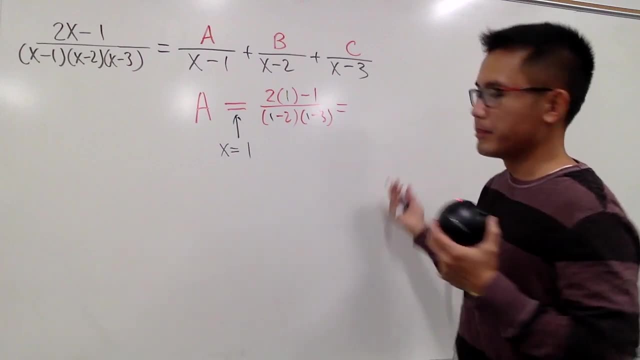 We're plugging 1 into here, so we will have 1 minus 2.. And then we're also plugging 1 into here, so we have 1 minus 3, like this, And then just do the computation. 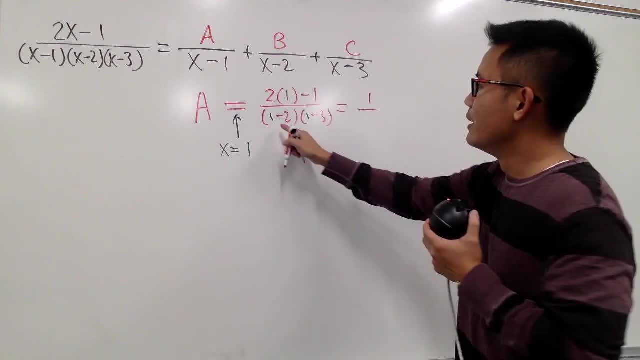 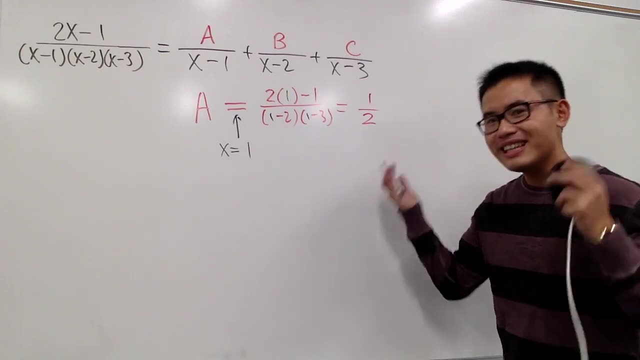 2 times 1 is 2, minus 1 is 1.. Over this is what? Negative 1 times negative, 2.. So all together, it's going to be positive 2. And that's it. That's the magic right. 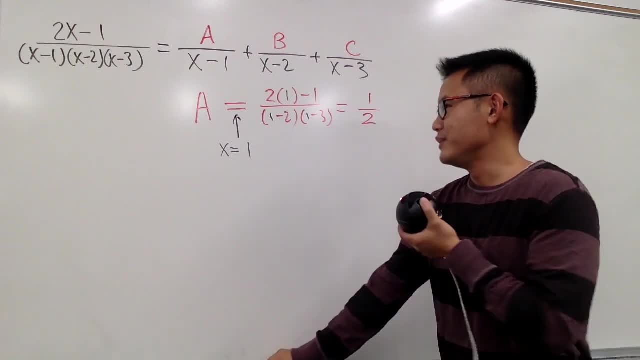 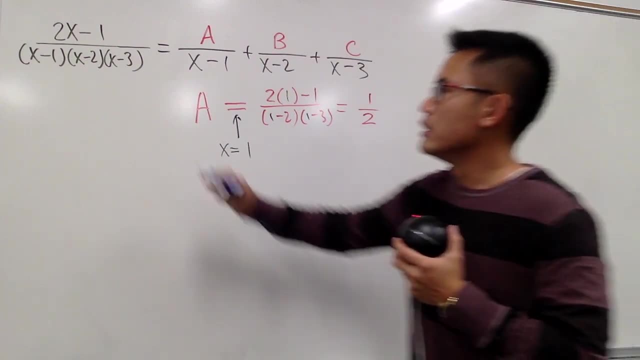 And now let me show you guys why it works. Of course, if you see this, you can also do the same for B and C, But let's just use A as an example. What we'll do is: this is a rational equation. 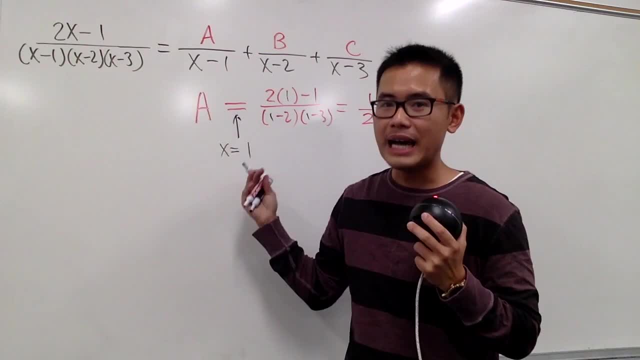 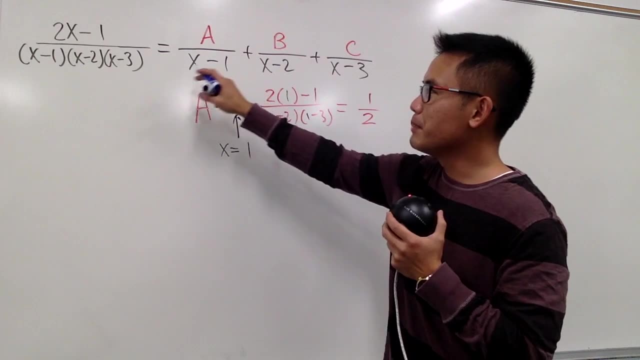 Usually we have to multiply everything by the lowest common denominator, namely all these three factors. But let's be smart. We are just going to multiply everything by this denominator, namely x minus 1 only. So let me do that right here for you guys, alright. 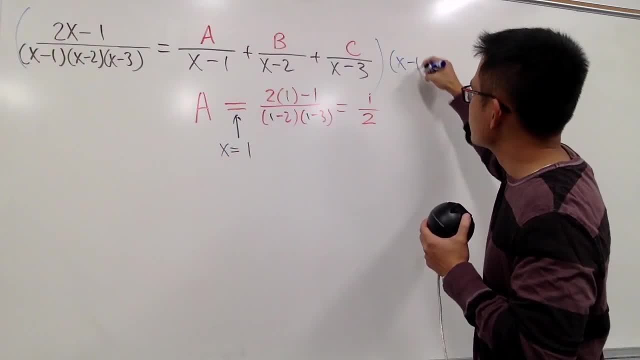 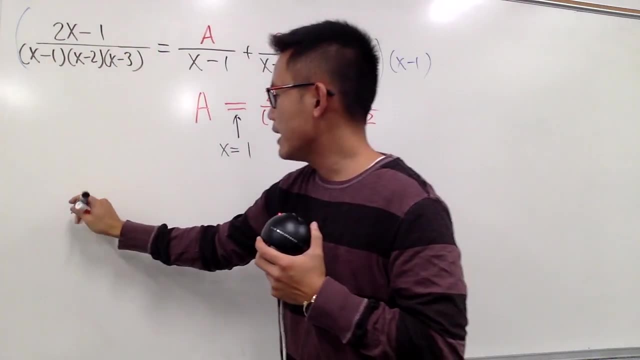 So multiply everything by x minus 1.. Just this. And now let's see what do we have This times? that We will just have 2x minus 1 over this and that cancel. That's why, as I told you, it didn't matter. 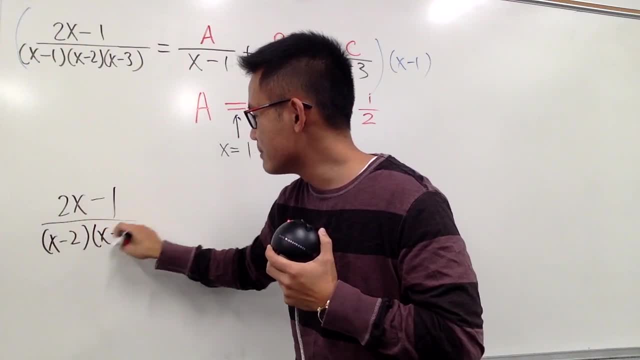 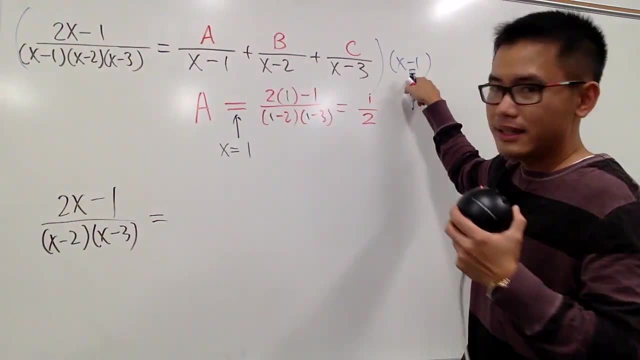 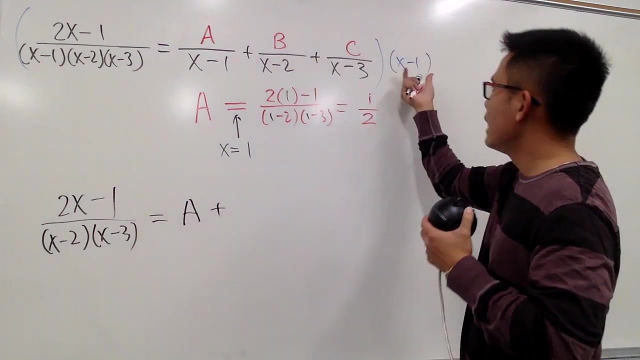 We will just have x minus 2 times x minus 3 now, isn't it- And this is equal to well, this fraction x minus 1 times this they cancel out. So we have just A and plus. well, this times that. 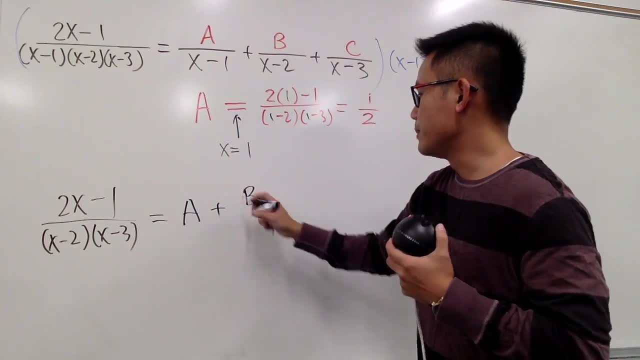 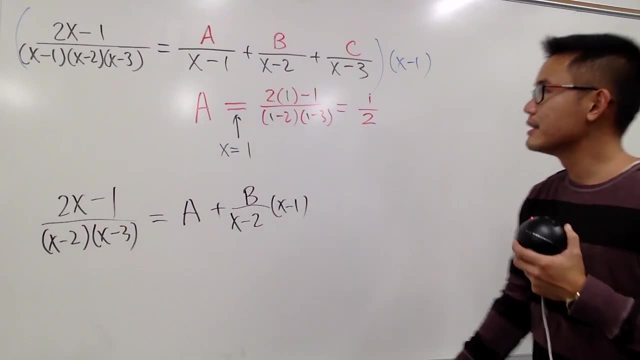 I will just put this on the top right, So we will have. well, just let me write it down: It's B over x minus 2 times x minus 1.. I don't want to multiply anything. alright, Once again for this right here, same thing. 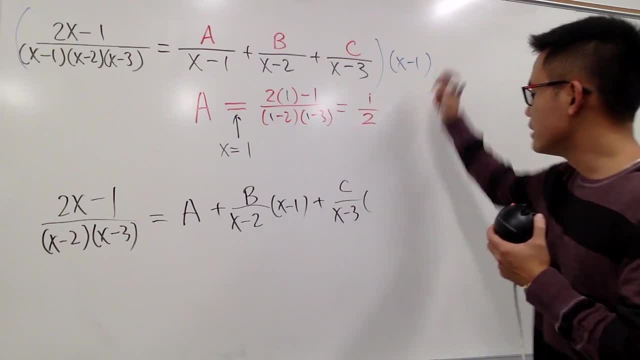 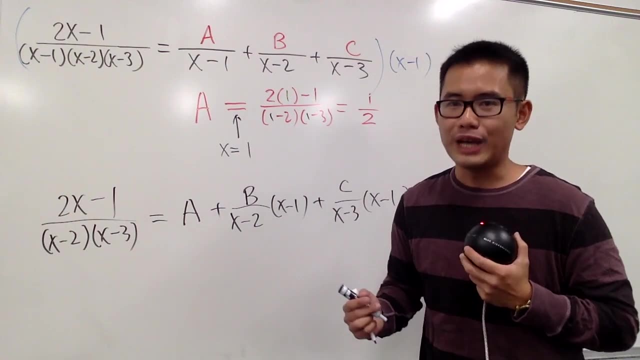 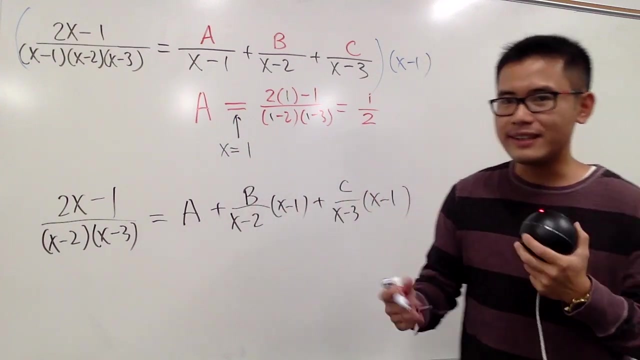 Plus Z over x minus, 3 times x minus 1, like this. And now this is the equation we have And how many variables we have: 4. Namely A, B, C and x. Technically, A B, C are the constants. 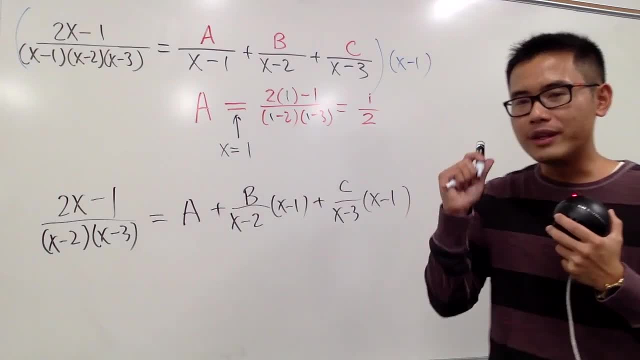 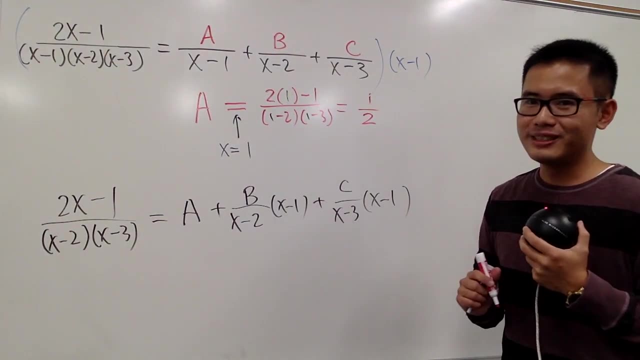 That's what we're trying to find out. x is the variable And we get to pick any value that we want for x. alright, And we are going to be smart And the best value for us to use is: x is equal to 1.. 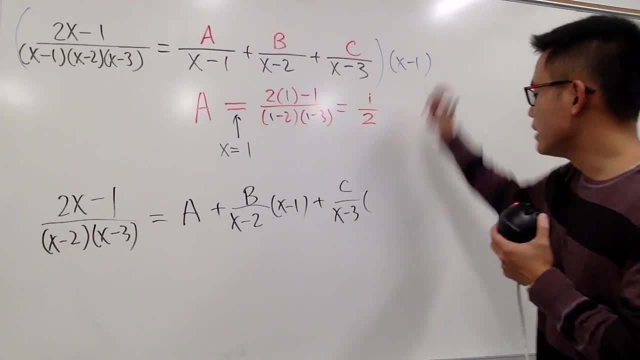 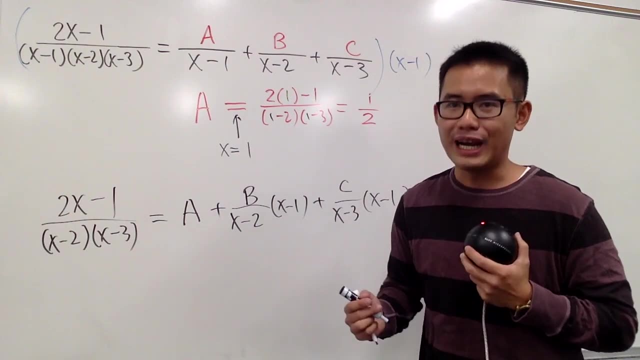 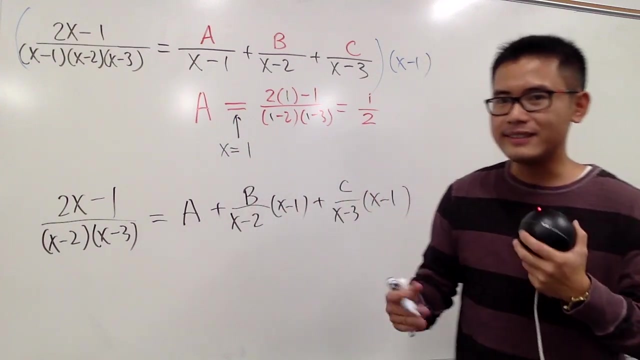 Plus C over x minus, 3 times x minus 1, like this. And now this is the equation we have And how many variables we have? 4, namely A, B, C and x. Technically, A B C are the constants. 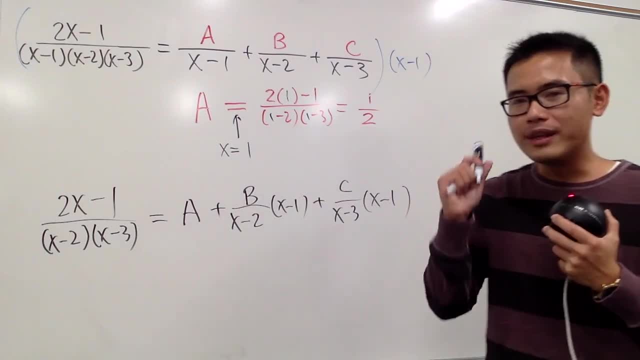 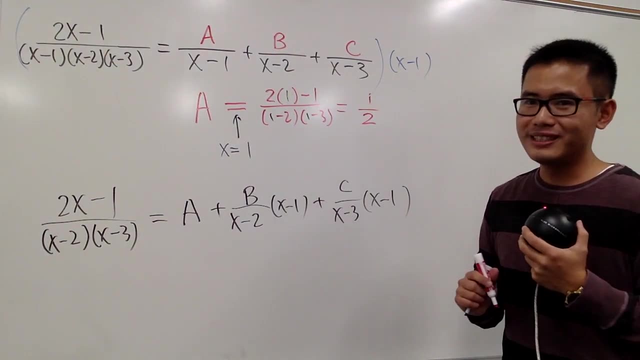 That's what we're trying to find out. x is the variable And we get to pick any value that we want for x. alright, And we are going to be smart And the best value for us to use is: x is equal to 1.. 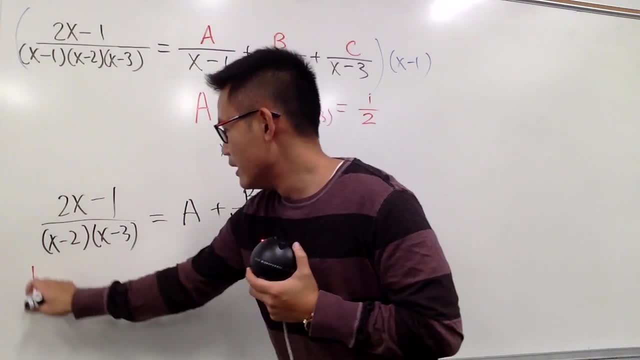 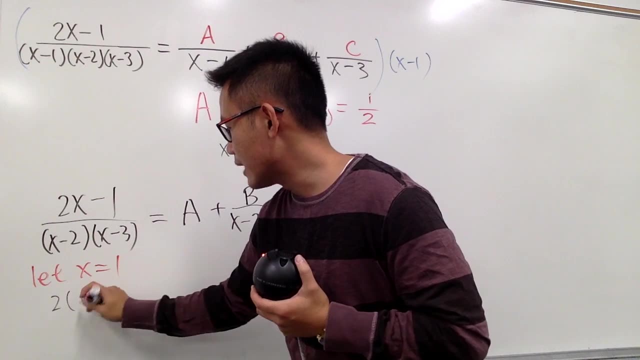 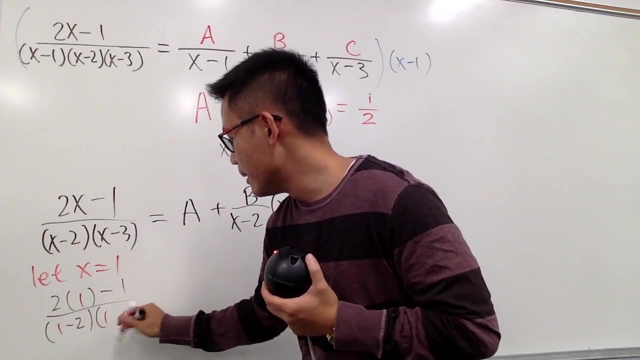 You will see why right now. So let me just show you guys all the work. alright, So let x equal to 1.. In this case, you see that I will just have to plug in 1 to here. So we have 2 times 1 minus 1 over 1 minus 2 times 1 minus 3, right? 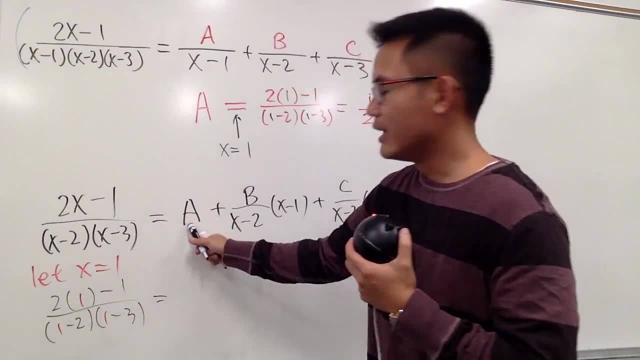 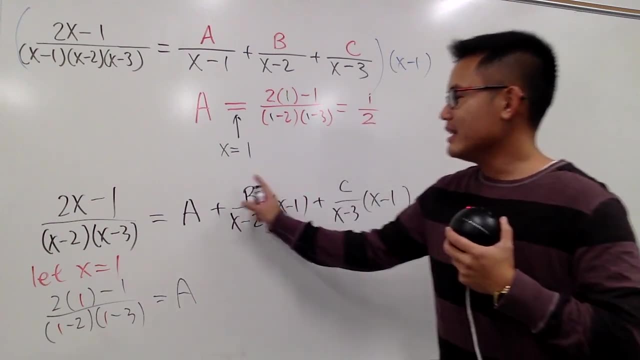 That's the left-hand side, And this is equal to aha. this is just A. A states A. But what happens when I plug in 1 into here? This may be hard, but 1 minus 1 is 0.. 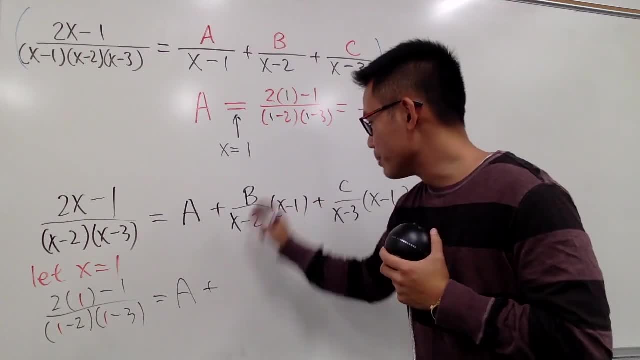 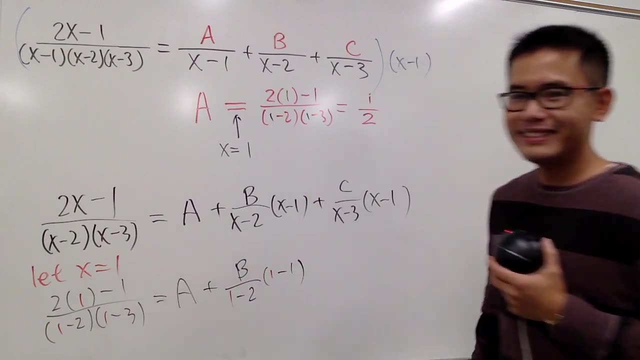 0 is going to kill this term, right, But I will still show you guys the work. We plus B over this is 10 equal to 1, minus 2 times 1 minus 1,. alright, This term is going to be 0.. 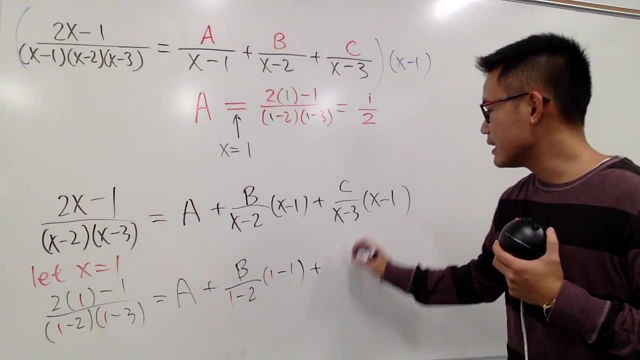 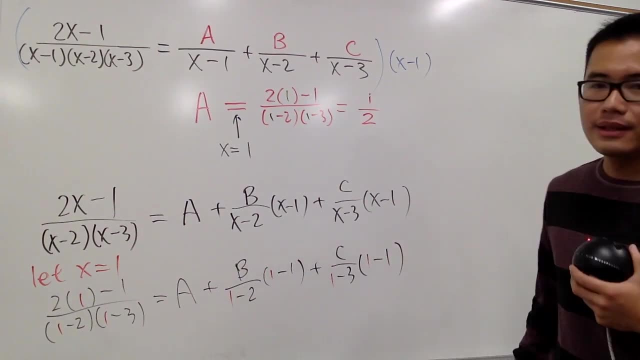 And in fact B doesn't matter. And likewise here plus C over 1 minus 3 times this x is 1, minus this 1, right, And as you can see, 1 minus 1 is 0.. This is going to kill this term. 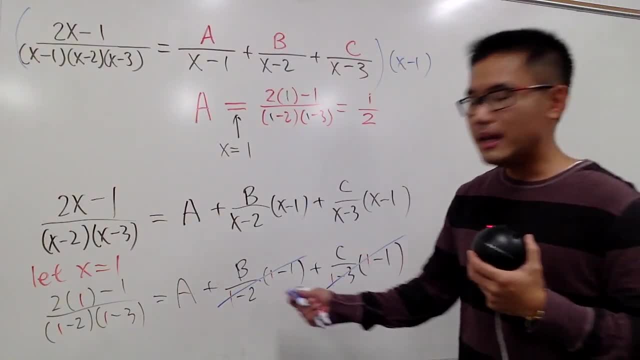 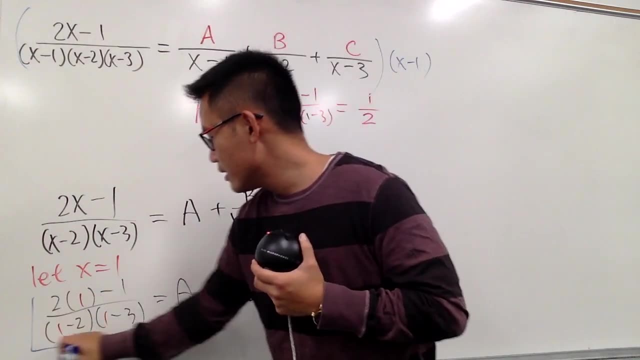 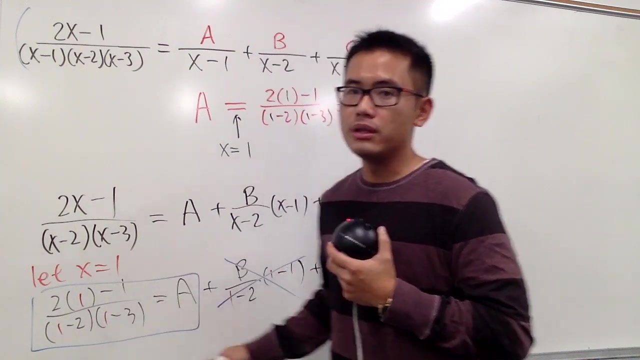 Likewise, 1 minus 1 is 0. It's going to kill this term. A is right here. B and C doesn't matter in plug-in, A right. So, as you can see, A is equal to 2 times 1 minus 1 over 1 minus 2 times 1 minus 3.. 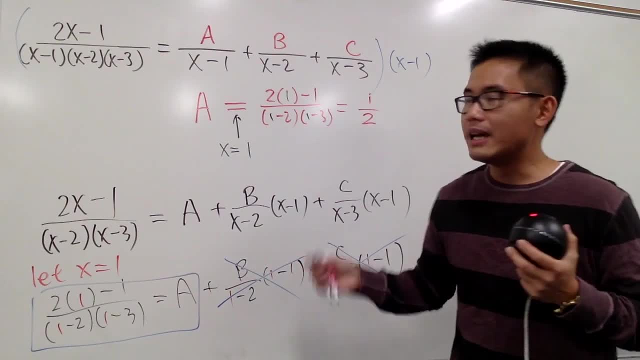 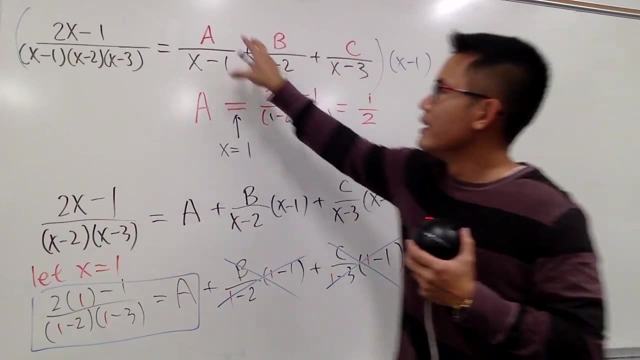 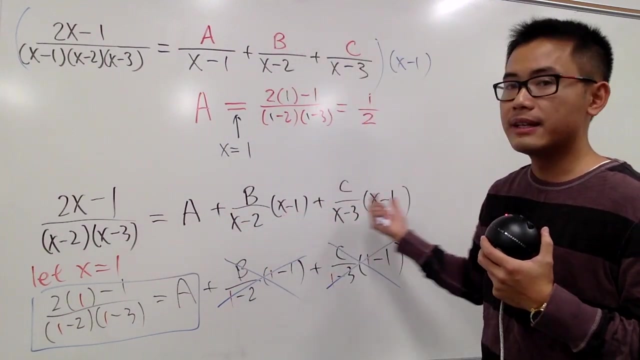 And that's exactly what we did earlier. So that's the process And this is the idea behind it. The idea is just that you multiply by this denominator only, so that this fraction will only have the top left and this other fraction will have this factor x minus 1.. 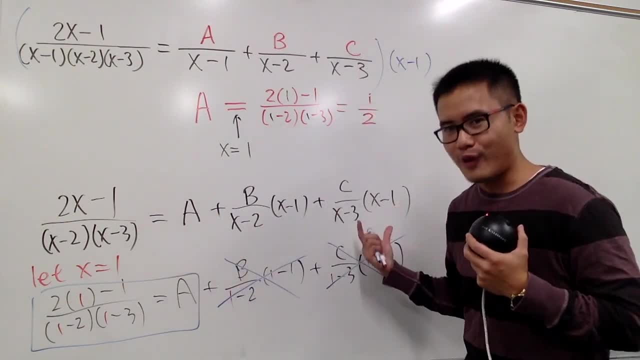 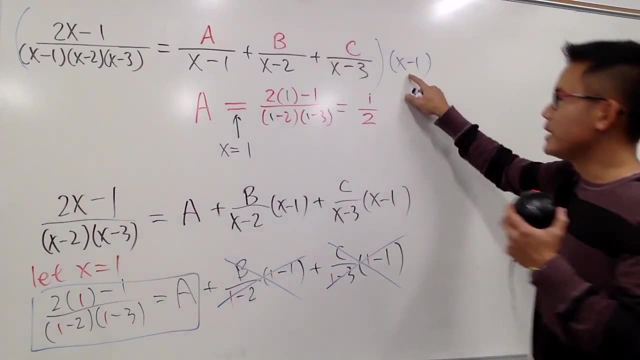 And the moment you plug in 1, you can kill these two fractions, so they don't matter. And be sure you cover up this right here, because x minus 1 is going to be cancelled with this. x minus 1, alright. 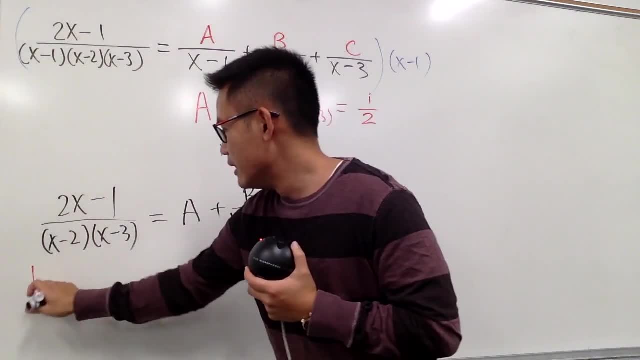 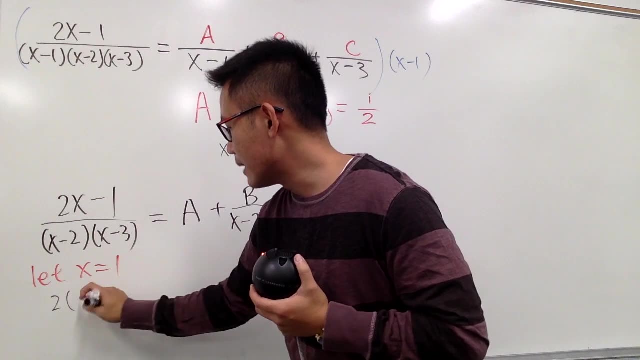 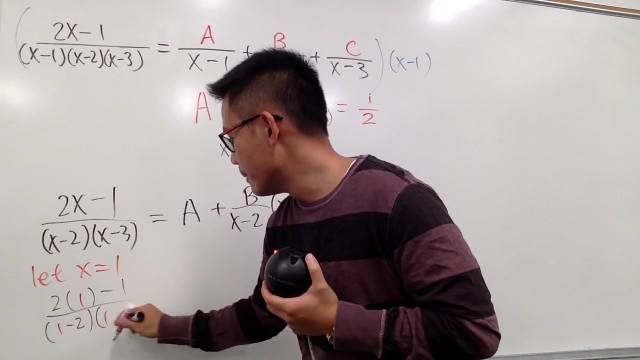 You will see why right now. So let me just show you guys all the work. alright, So let x equal to 1.. In this case, you see that I will just have to plug in 1 to here. So we have 2 times 1 minus 1 over 1 minus 2 times 1 minus 3, right? 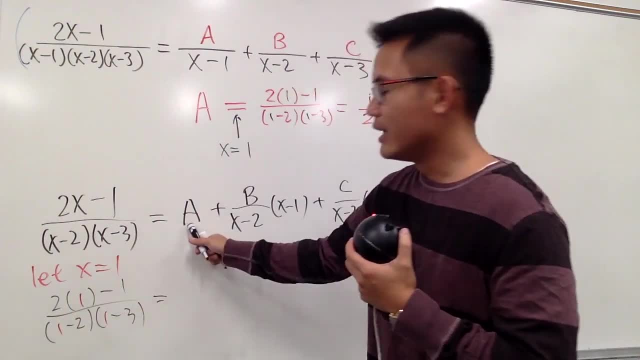 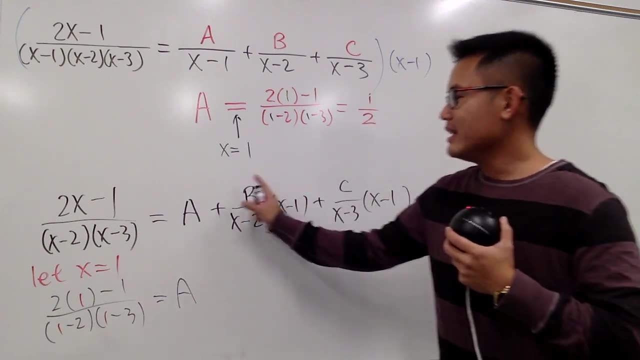 That's the left-hand side, And this is equal to aha. this is just A. A states A. But what happens when I plug in 1 into here? Uh, this may be hard, but 1 minus 1 is 0.. 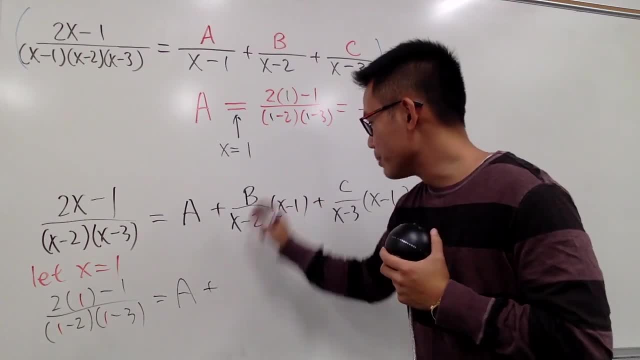 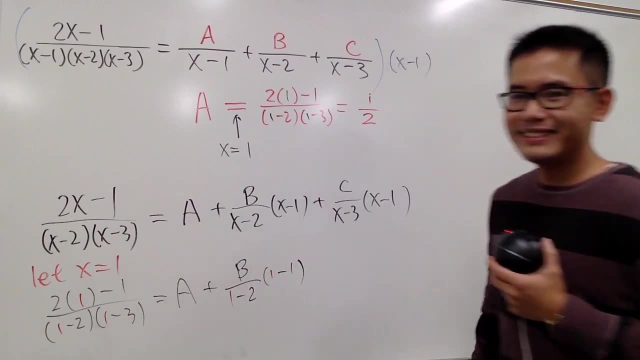 0 is going to kill this term, right, But I will still show you guys the work. We plus B over this is 10 equal to 1 minus 2 times 1 minus 1, alright, This term is going to be 0.. 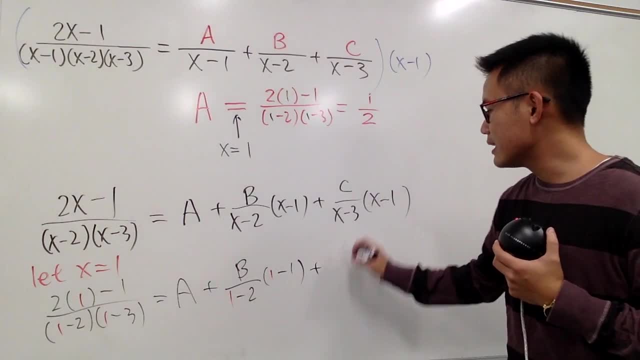 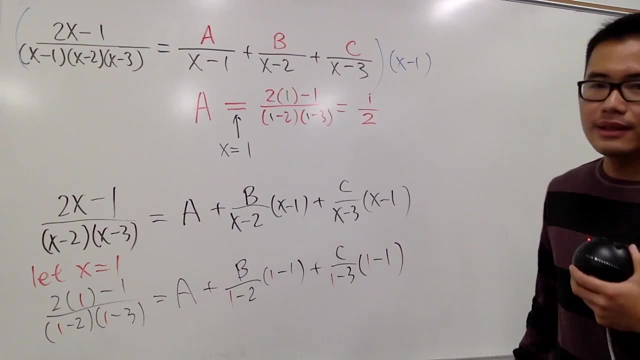 And in fact B doesn't matter. And likewise here plus C, over 1 minus 3 times this x is 1 minus this 1, right, And as you can see, 1 minus 1 is 0, this is going to kill this term. 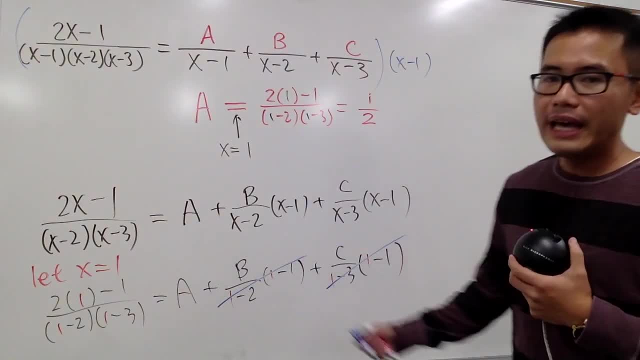 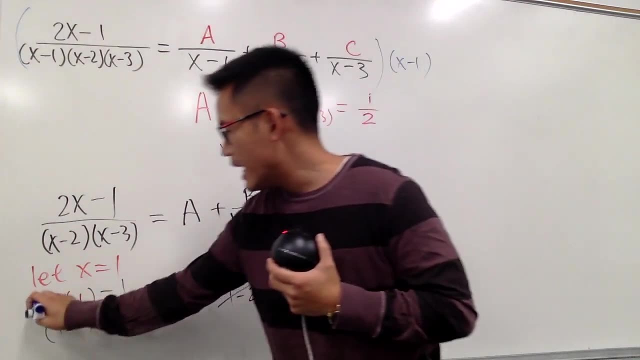 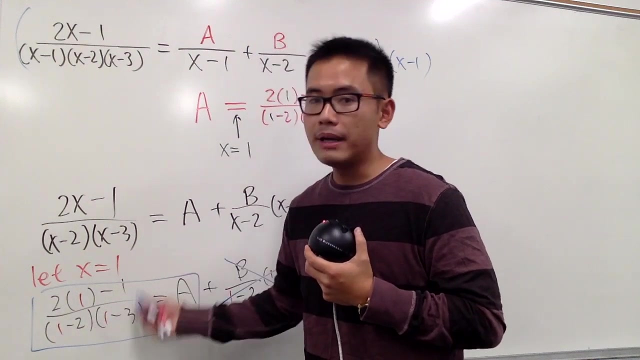 Likewise, 1 minus 1 is 0, it's going to kill this term. A is right here. B and C doesn't matter in plug-in A right. So, as you can see, A is equal to 2 times 1 minus 1 over 1 minus 2 times 1 minus 3.. 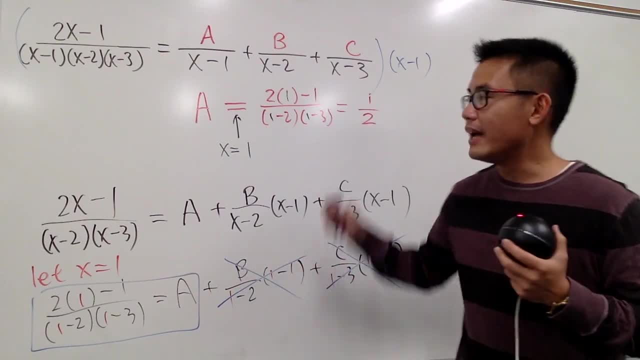 And that's exactly what we did earlier. So that's the process and this is the idea behind it. The idea is just that you multiply by this denominator. So that's the process and this is the idea behind it. The idea is just that you multiply by this denominator. 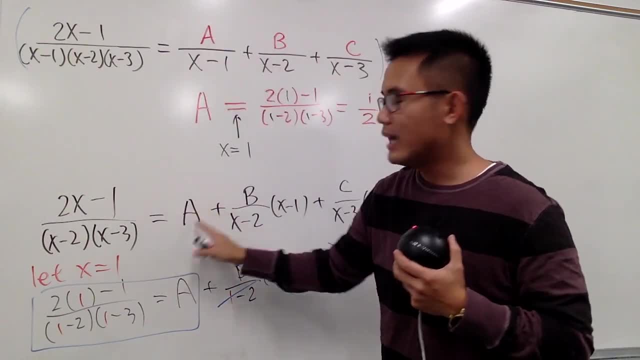 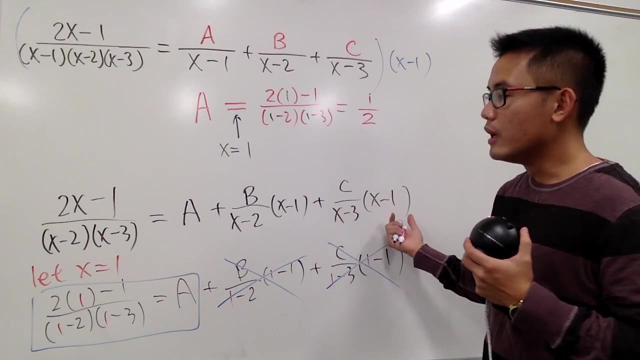 The idea is just that you multiply by this denominator Only, so that this fraction will only have the top left and these other fractions will have this factor x minus 1.. And the moment you plug in 1, you can kill these two fractions. 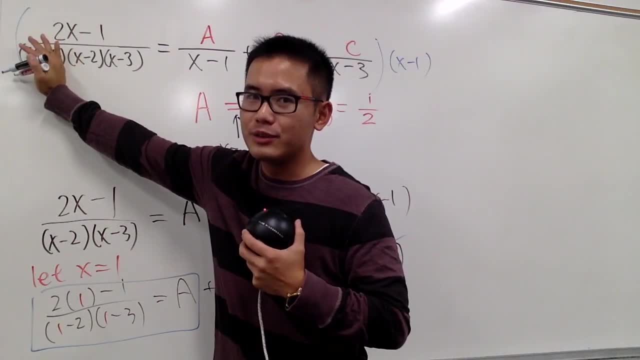 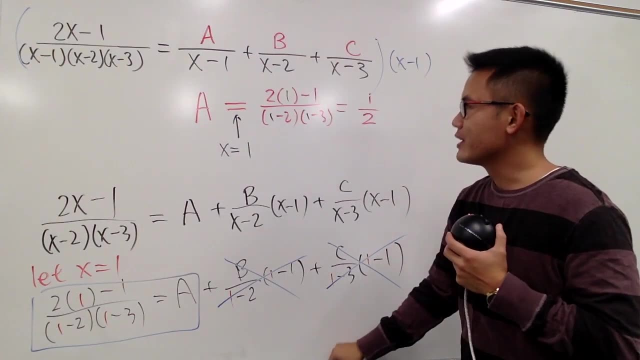 So they don't matter, And be sure you cover up this right here, because x minus 1 is going to be cancelled with this x minus 1, alright, And now, since we got A already, as I said, I'm just going to show you guys B and C with a cover-up. 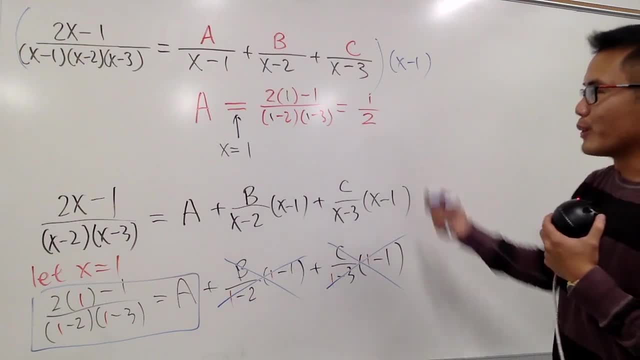 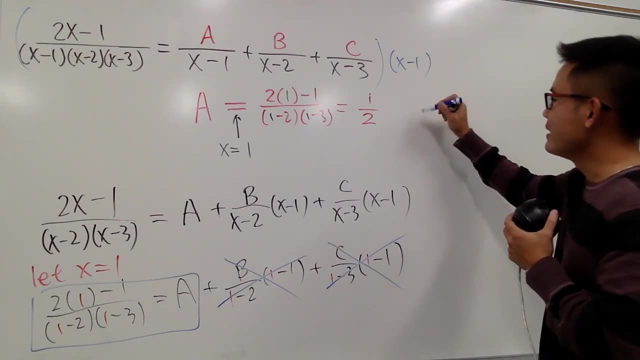 And now, since we got A already, as I said, I'm just going to show you guys B and C with a cover-up method, because it's meant to be really, really easy. alright, It's decided so that. So we can be really really happy. 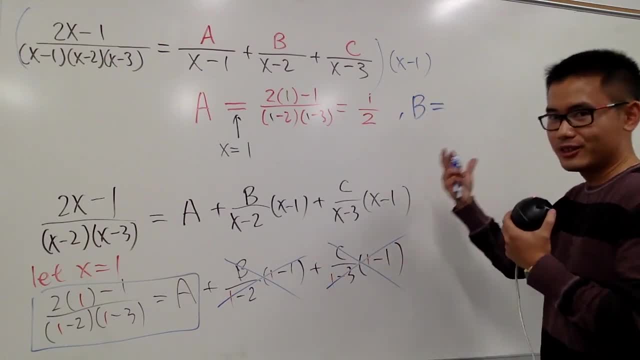 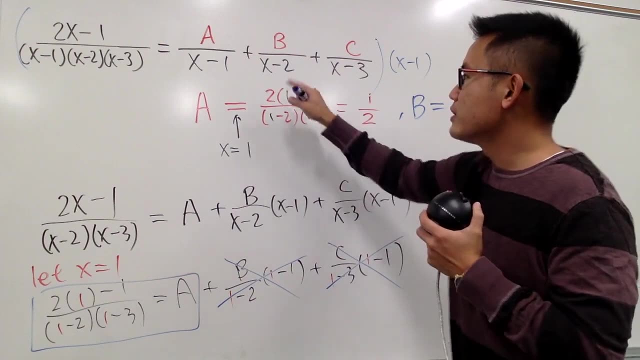 Let's figure out what B is, And I'm not going to do this work because you guys know this is going to be quick B: it has the x minus 2 under the denominator, right here, right? So to figure out B I will have to plug in: x is equal to what? 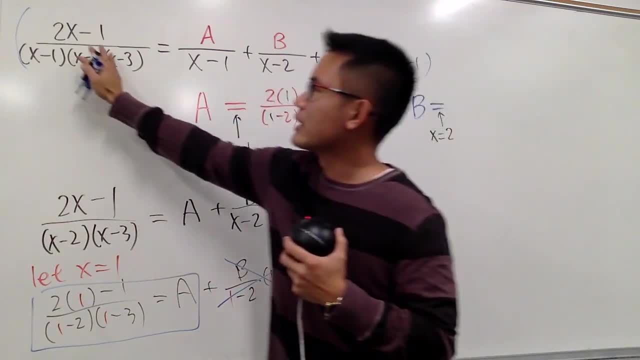 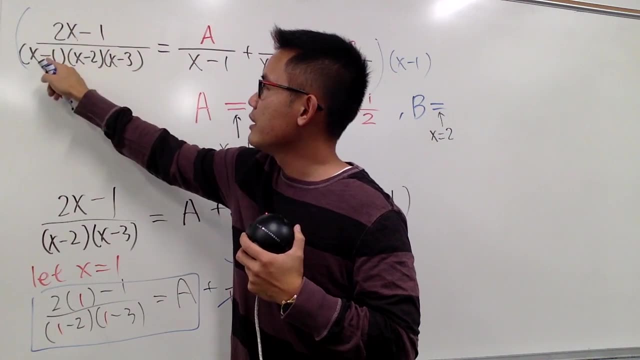 2,. okay, I'll come back to the original cover this up: the x minus 2.. And to make x minus 2 equal to 0, x has to be 2.. And now plug in 2 into here, here and here, right. 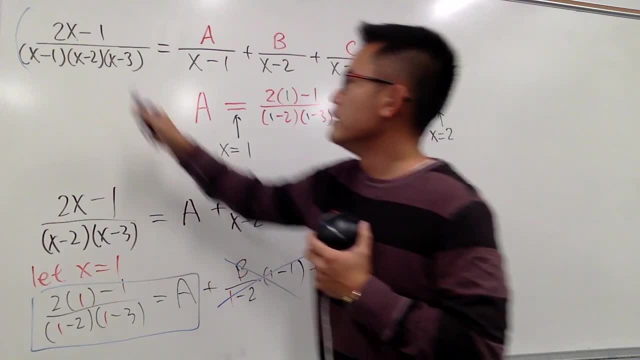 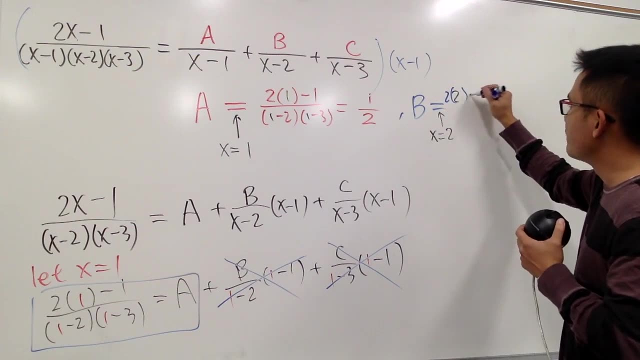 These two factors, the fractions don't matter anymore. Anyway, we have 2 times x and x is the 2, so we'll have the 2 times 2 like this: this is the x value and then minus 1 over. plug in 2 into this x and that x. 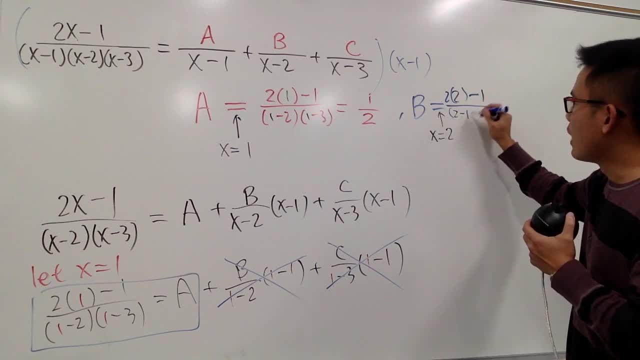 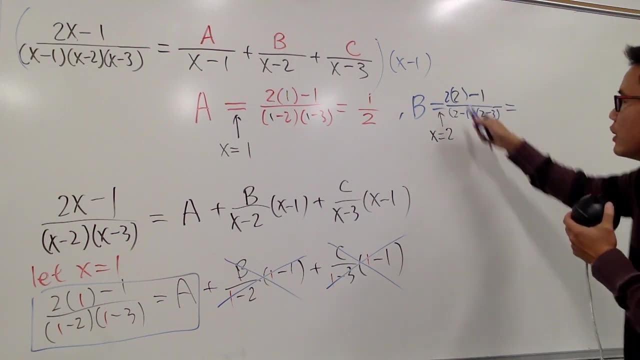 so we will have 2 minus 1 times 2 minus 3, right, And just work this out: 2 times 2 is 4,, 4 minus 1 is 3 over, 2 minus 1 is 1, and 2 minus 3 is negative 1,. 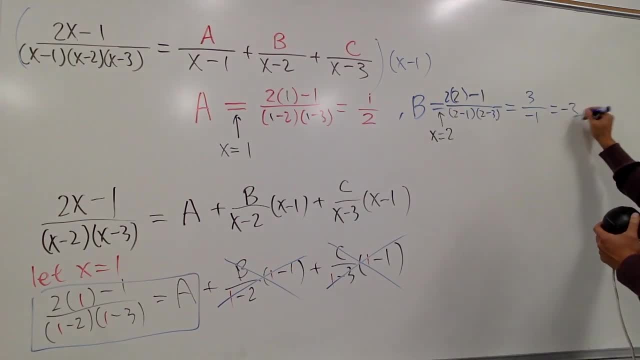 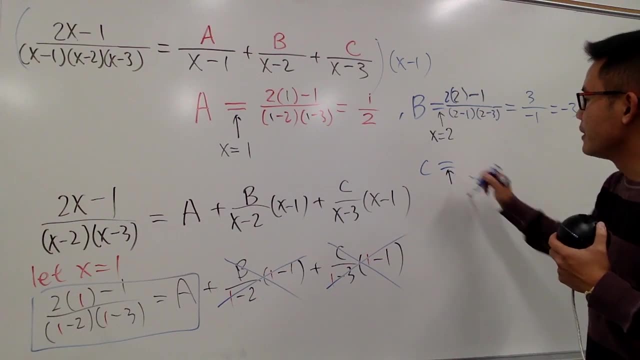 so we have 1 times negative 1, so we have negative 1, so together it's going to be negative 3.. And let's put down c right here, right c. I have to pick out the x value. 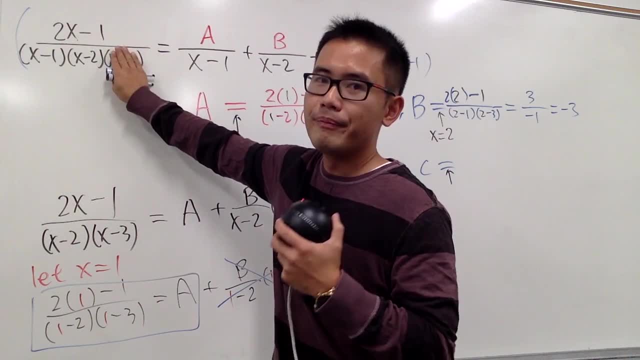 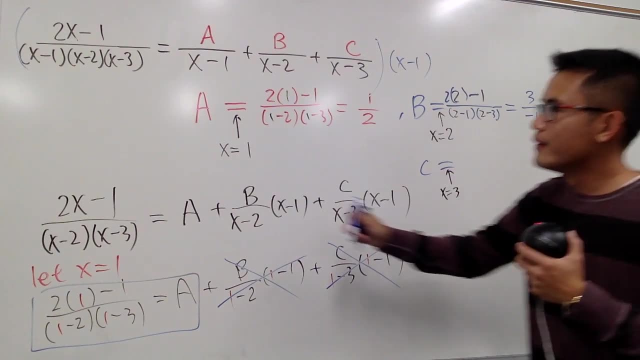 This is c over x minus 3.. Come here, cover this up. How can I make this equal to 0?? x has to be 3.. So plug in x equal to 3.. This, this and that, so we will have 2 times 3,. 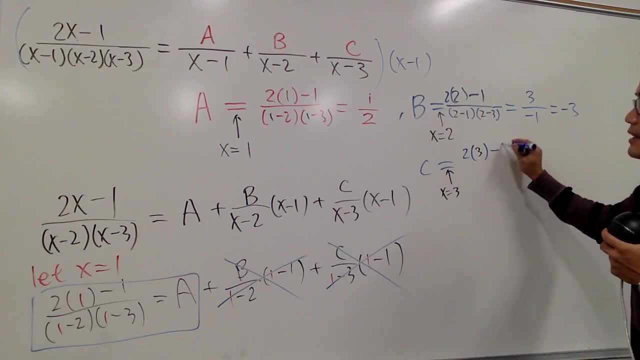 so we have 2 times 3 minus 1 over plug in 3 here and here, right. So we have 3 minus 1 times 3 minus 2, like this, and at the end just do the work: 2 times 3 is 6, minus 1 is 5, over this is 2, this is 1,. 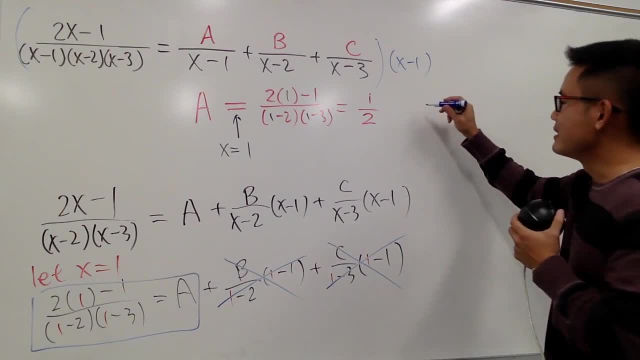 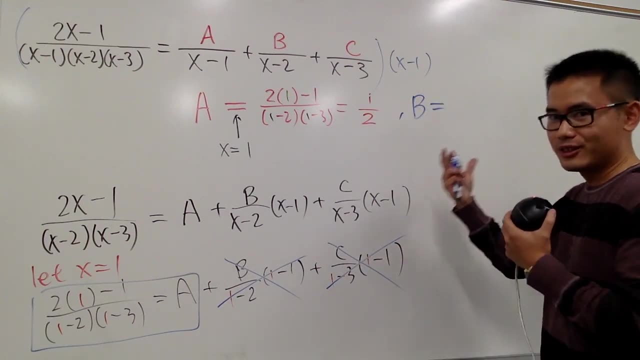 method because it's meant to be really really easy. alright, it's designed it so that we can be really really happy. let's figure what B is, and I'm not going to do this work because you guys know this is going to be quick. B: it has the X minus. 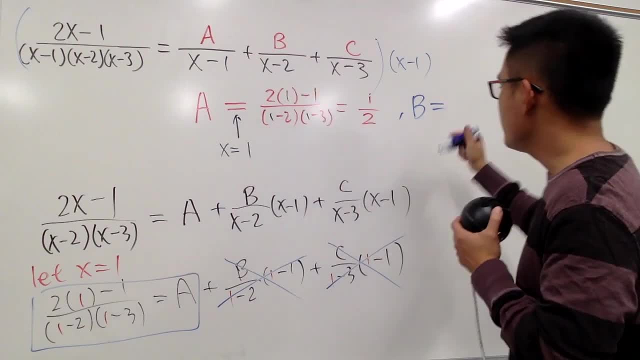 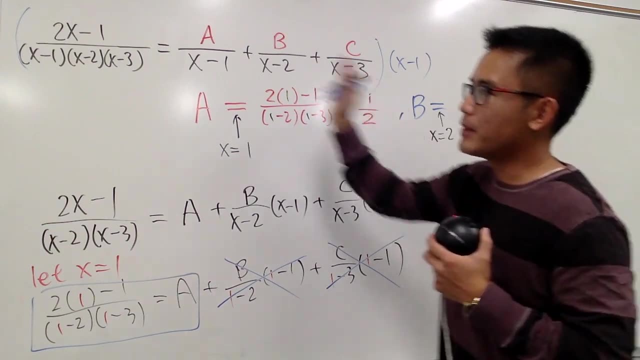 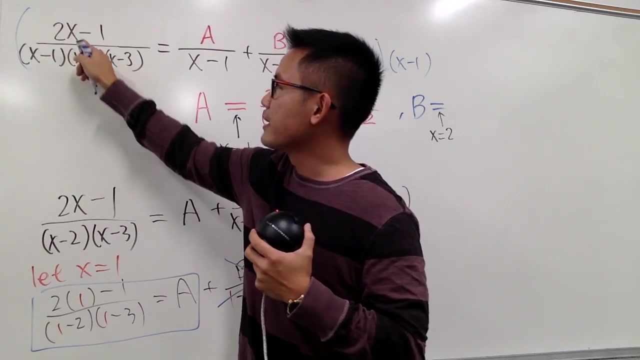 2 under the denominator right here. right? so to figure out B I will have to plug in: X is equal to what? 2? okay, I'll come back to the original cover this up: the X minus 2. and to make X minus 2 equal to 0, X has to be 2, and now plug in 2 into. 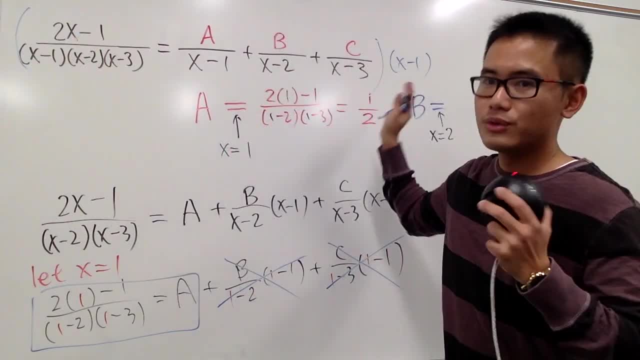 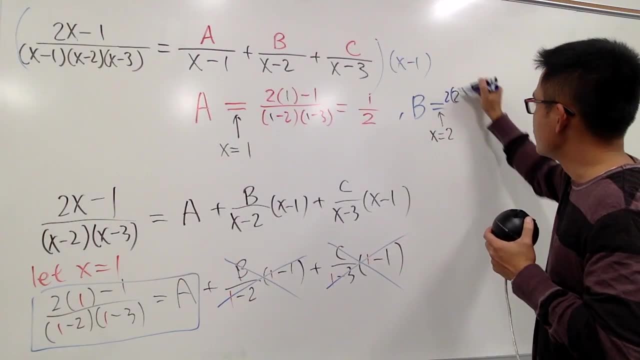 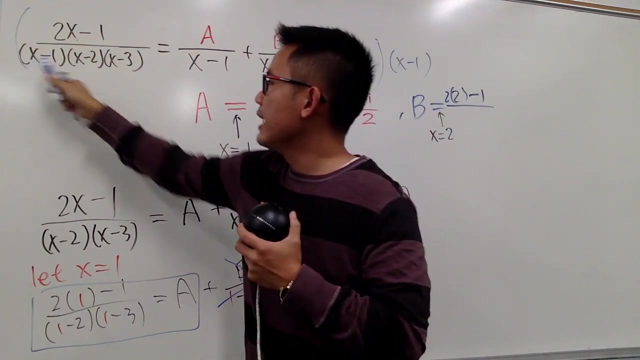 here, here and here. right these two factors. the fractions don't matter anymore. anyway, we have 2 times X and X is the 2. so we'll have the 2 times 2 like this: this is X value and then minus 1 over. plug in 2 into this X and that X. so 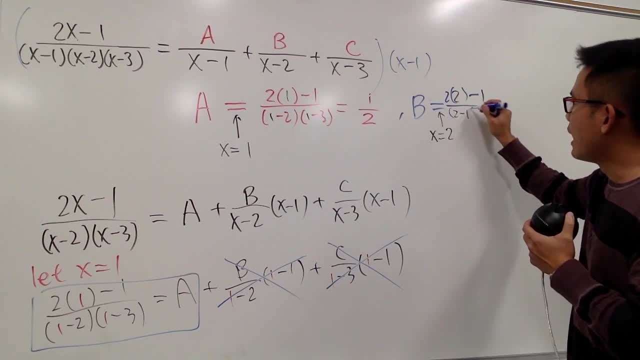 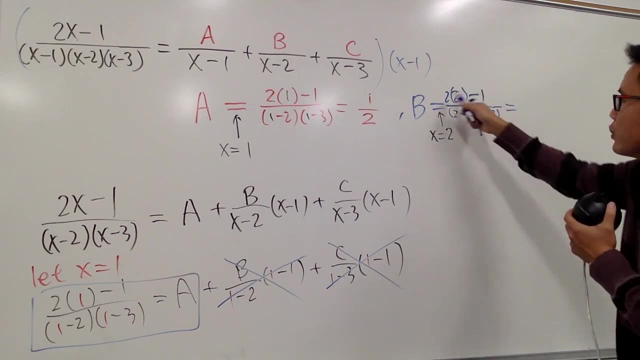 we will have 2 minus 1 times 2 minus 3, right, and just work this out: 2 times 2 is 4, 4 minus 1 is 3 over. 2 minus 1 is 1 and 2 minus 3 is negative 1. so we have 1 times negative 1, so 1 negative 1, so 2. 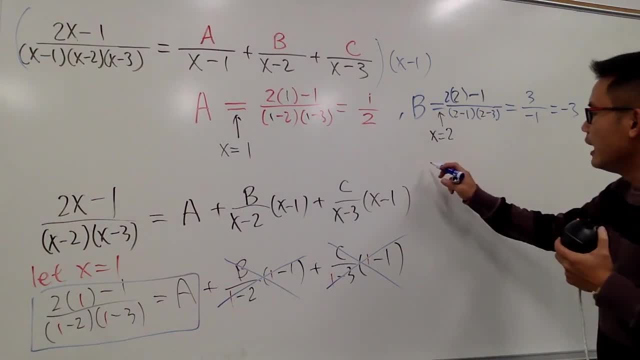 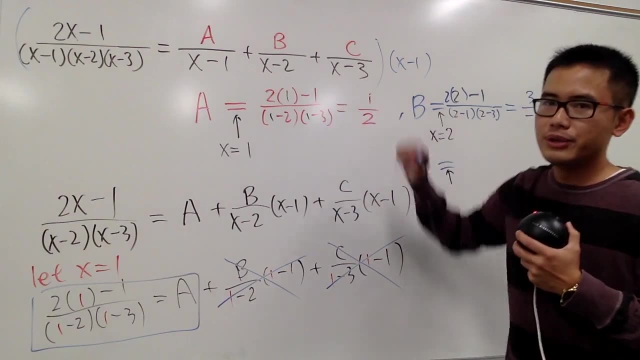 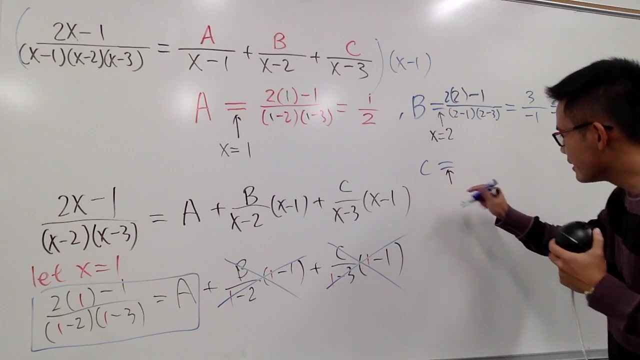 together it's going to be negative 3. and let's put on C, right here, right C. I have to pick out the X value. this is C over X minus 3. come here, cover this up. how can I make this equal to 0? X has 3, 3. so plugging X equal to 3 for this, this and 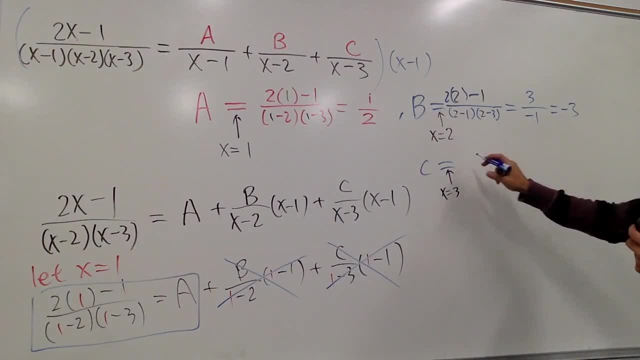 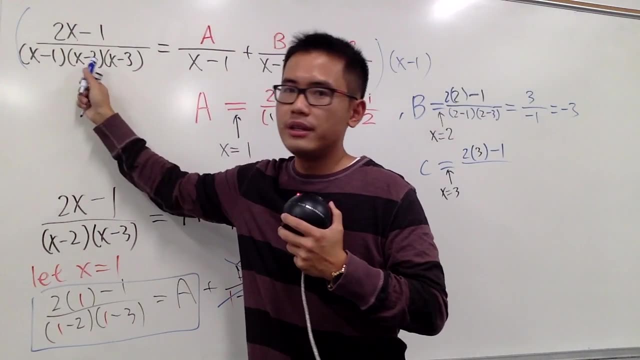 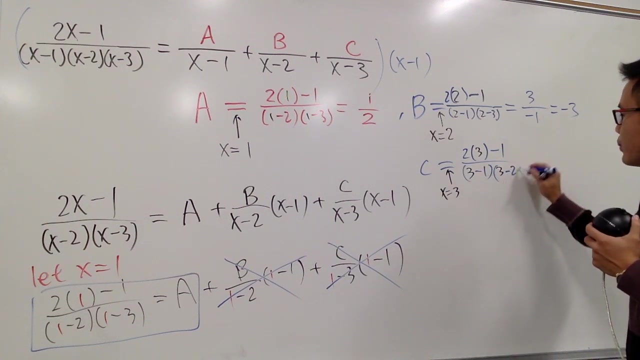 that. so we will have 2 times 3. so we have 2 times 3 minus 1 over plug in 3 here and here, right, so we have 3 minus 1 times 3 minus 2, like this, and at the end just do the work. 2 times 3 is 6 minus 1. 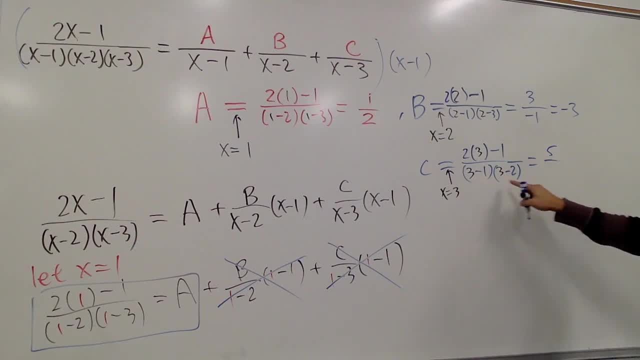 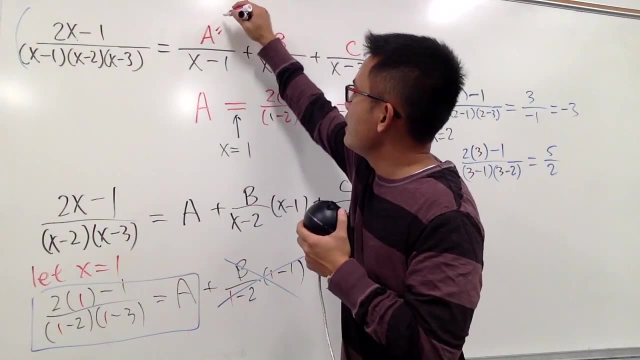 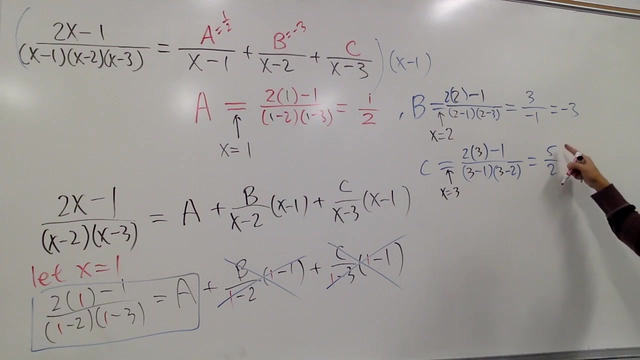 5 over. this is 2, this is 1, so 2 times 1 is 2. so we are done right, and usually I just like to do this for you guys: a is 1 half and B is negative 3 and C is 5 over. 2 right.